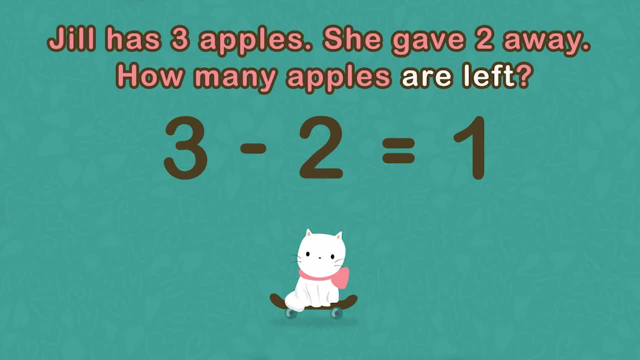 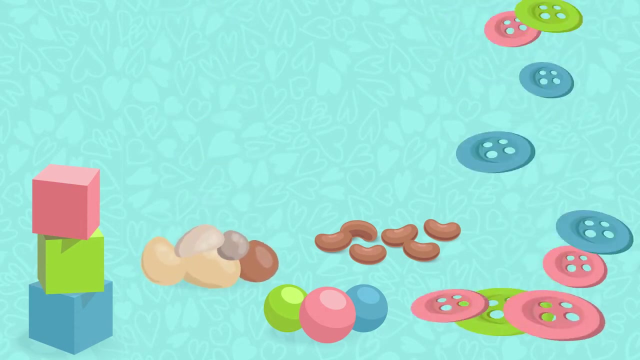 is a clue that you must subtract to find how many remain after a part has been taken away. Using objects to count is a helpful strategy for solving subtraction problems. Any objects will work, but cubes, beads, dried beans, pebbles and buttons make great counters. 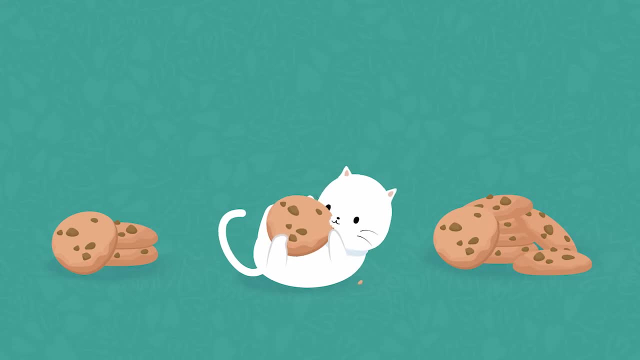 You can even use cookies to solve subtraction problems. Just try not to eat your cookie counters before you solve all the problems. This subtraction problem is 5 minus 2.. Use the cookies as counters. Begin with 5.. 1,, 2,. 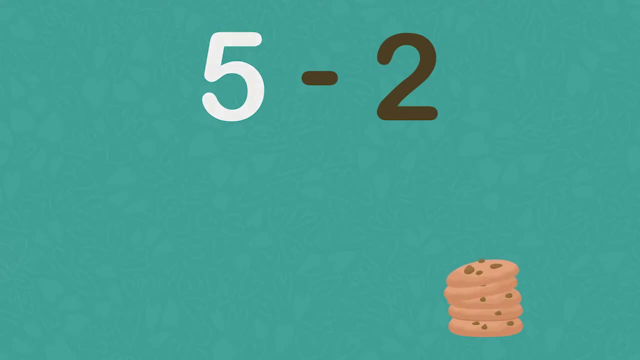 3,, 4, 5.. The next part of the problem is minus 2.. This means you must take away 2.. Take 2 cookies away from the 5.. 1, 2. Remember not to eat the cookies You have. 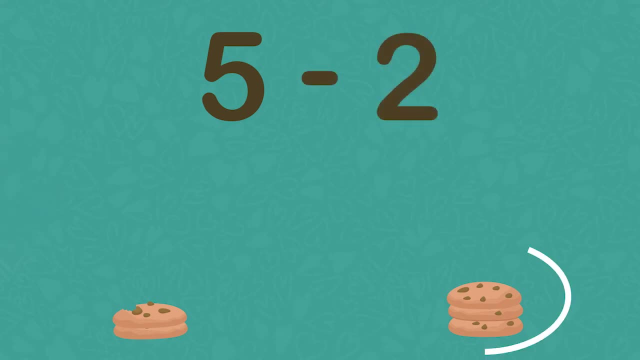 more problems to solve. How many cookies are left? Count to find the difference: 1,, 2, 3.. 3 cookies are left. The solution to the problem is 3.. The next subtraction problem is 8 minus 5.. Count out 8 cookies to start: 1,, 2,, 3,, 4,, 5,, 6, 7, 8.. The problem says: 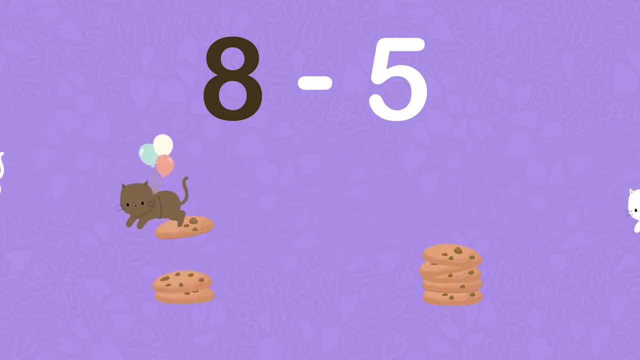 to take away 5.. 1,, 2,, 3,, 4, 5.. How many are left? Count the remaining cookies: 1, 2, 3.. 8 minus 5 equals 3.. 3 is the difference. 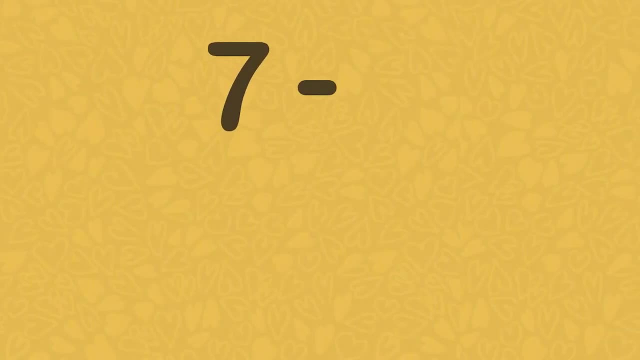 Now use the cookies to solve this problem: 7 minus 3.. Count out the total of 7 cookies to begin: 1,, 2, 3, 4, 5.. 1,, 2,, 3,, 4, 5.. 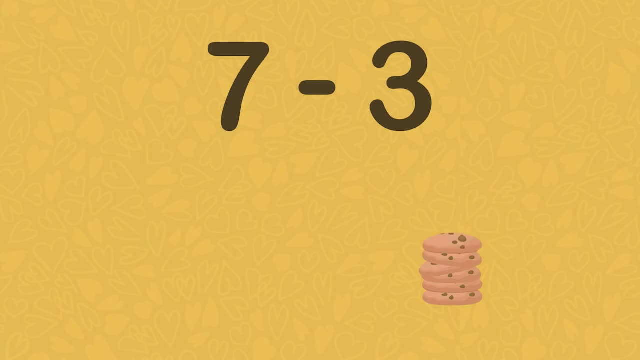 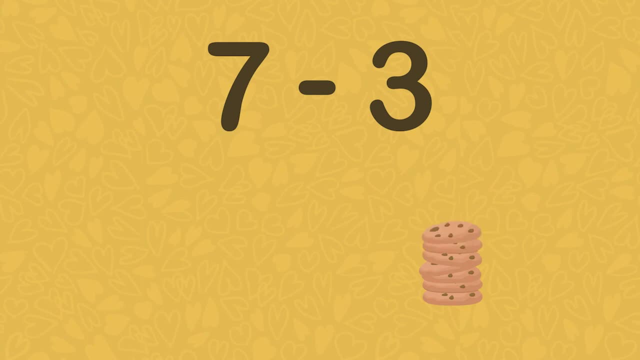